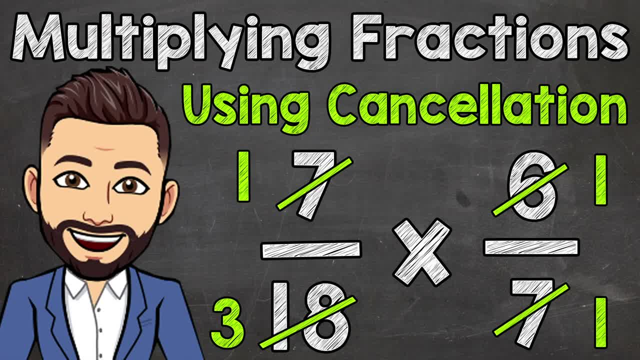 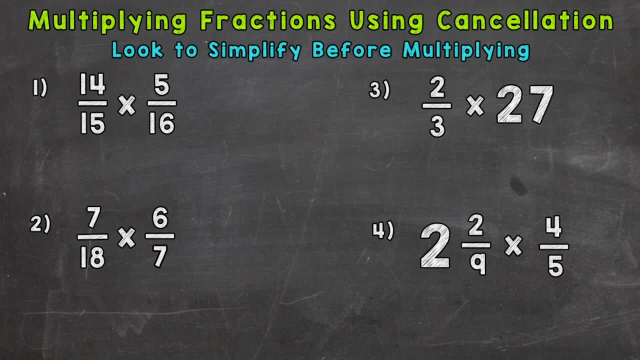 Welcome to Math with Mr J. In this video, I'm going to cover how to multiply fractions using cancellation, And cancellation is a way to simplify fractions before we multiply. This gives us smaller and easier numbers to work with. Understanding and using cancellation can make problems a lot simpler. 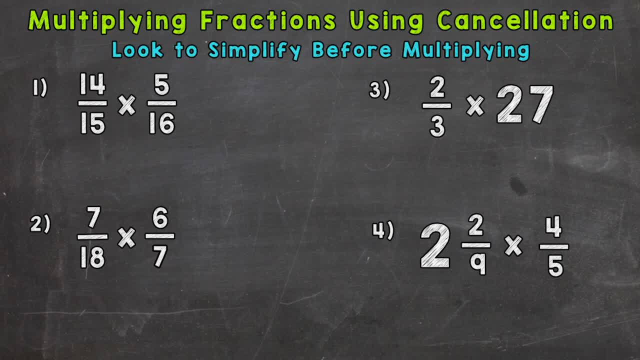 and easier to work through. So let's get into our four examples here and start with number one, where we have 14, 15 times 5, 16.. What we need to do first is look for common factors between the numerators- the top numbers here- and the denominators, so top and bottom. We are not looking for common factors. 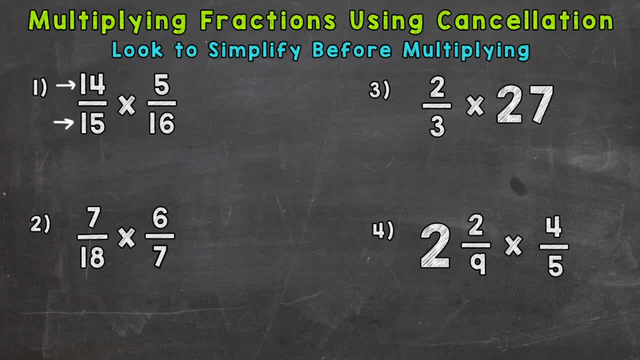 horizontally or side to side, so always top and bottom. Think of it like simplifying fractions, but you can use all of the numbers within the problem. So, for example, looking for common factors here, I know that 15 and 5 have a common factor of 5.. So let's divide both 15 and 5 by that common factor of 5.. 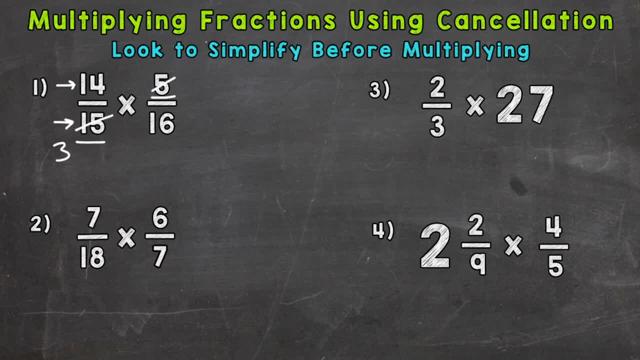 15 divided by 5 is 3.. 5 divided by 5 is 1.. Let's take a look at 14 and 16 to see if they have any common factors besides 1.. And they do. They have a common factor of 2.. So let's divide both of those by 2.. 14 divided by 2 is 7.. 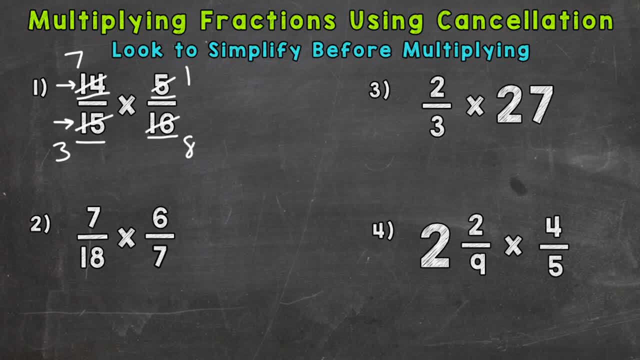 16 divided by 2 is 8.. So I'm going to rewrite my problem here. and we have 7 over 3 times 1 over 8 and we multiply fractions by going straight across, so we get 7- 24ths. Always check to see if we can simplify further here, but 7- 24ths is. 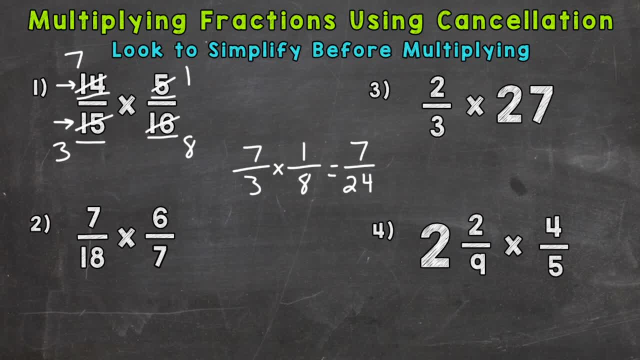 in simplest form. the only common factor between 7 and 24 is 1. so we are done. So you can see that we got much simpler and easier numbers to work with compared to the original problem. So let me rewrite the original problem here: 14, 15ths times. 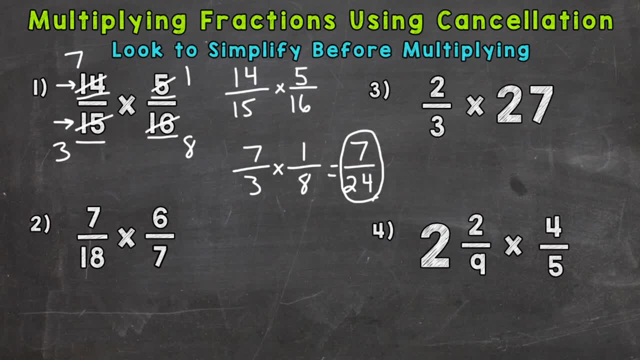 5 16ths. So 14 times 5 is going to give us 70 and 15 times 16 is going to give us 240.. So you can see that those multiplication problems there are a little more complex and the numbers are greater in value than our cancellation. 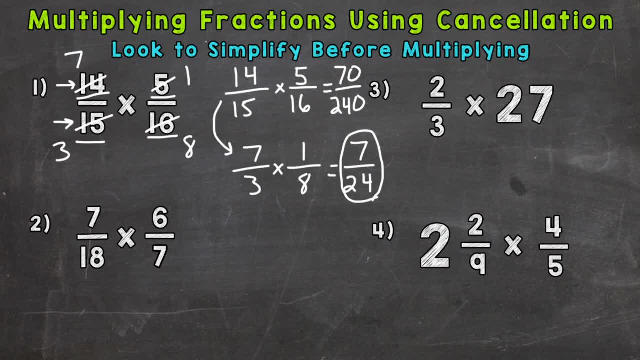 version there of 7 over 3 times 1 over 8 and also 70 over 240. that's going to take a lot more simplifying and work there. So you can see that the cancellation made everything simpler. Now 70 over 240 is equivalent to: 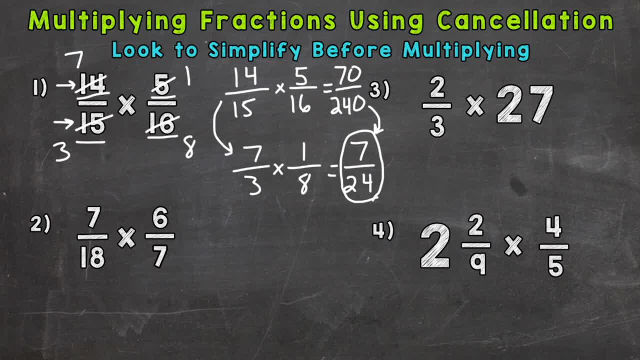 what we got with the cancellation. We would just need to simplify that and break that down and it would eventually get to 7- 24ths. On to number 2, where we have 7 18th times 6 7ths. So we need to look at numerators and denominators top. 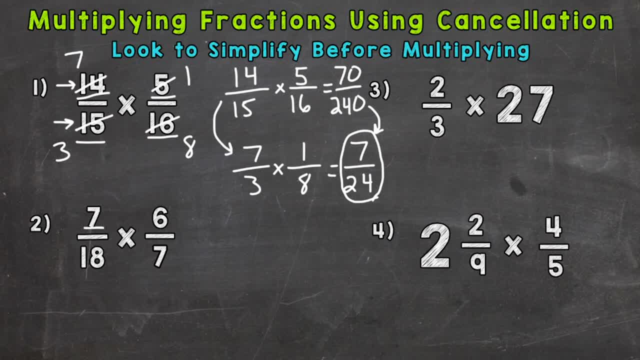 and bottom, and we can see that we have a 7 and a 7 here, So a common factor of 7 between those 7s. So divide each by 7 and we get 1.. 7 divided by 7 is 1.. All right, let's take a look at 18 and 6 here. So do we have any common? 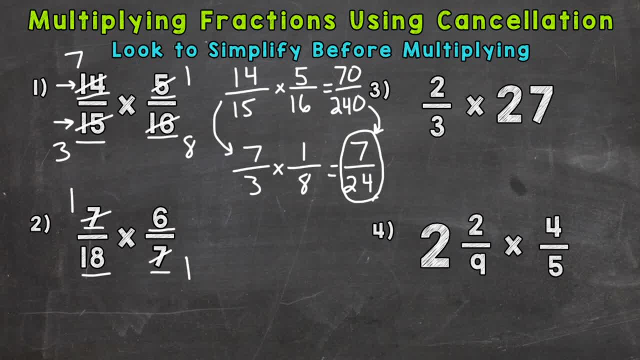 factors Yes, 2, 3 and 6.. Let's use the greatest common factor of 6.. That way we have less simplifying in the end once we get our answer. If you don't use the greatest common factor between two numbers, that's fine, You're just going to. 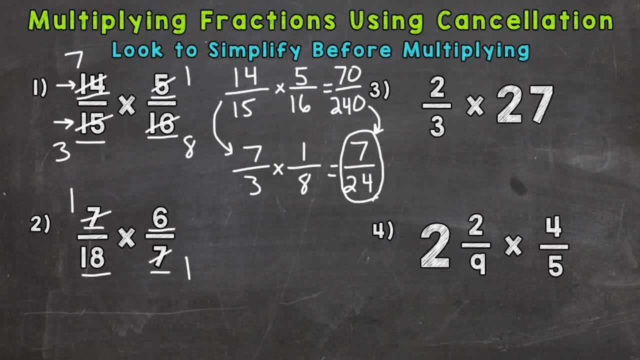 have more simplifying in the end. So we'll divide 18 and 6 by 6. So 18 divided by 6. 6 is 3 and 6 divided by 6 is 1.. So we end up with 1 over 3 times 1 over 1.. And 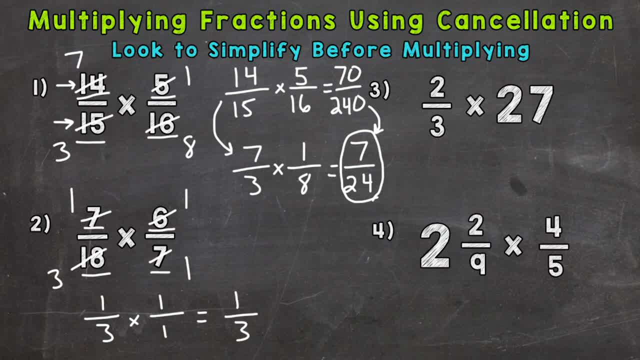 that's going to get us 1, 3rd, And 1, 3rd is in simplest form. So we are done. Now again, you can do 7, 18ths, times 6, 7ths, and keep it as is, And you will get the. 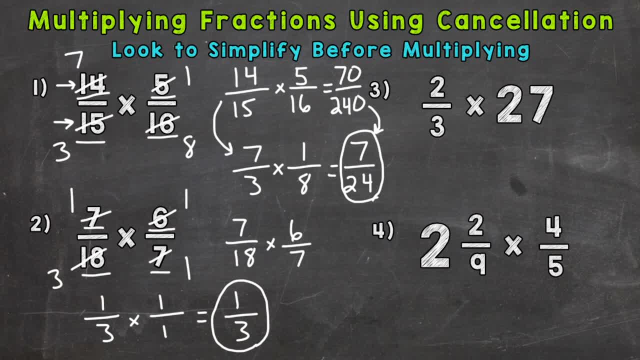 same answer. It's just going to take more simplifying at the end there. And you do have larger numbers in value to work with: 7 times 6 and 18 times 7.. So on to number 3, where we have 2 3rds times 27.. 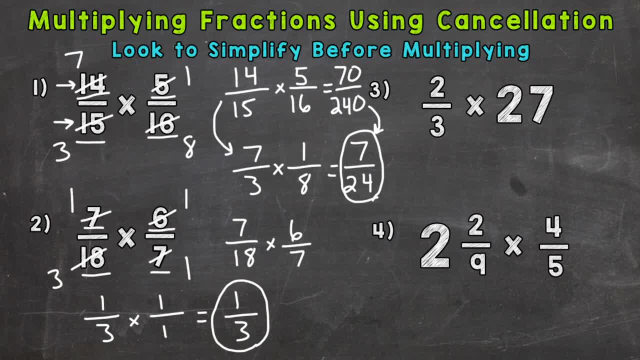 So a fraction times a whole number. What we need to do here is write 2 3rds and we need to make 27 into a fraction. so we have a numerator and a denominator And all we need to do if we have a whole number, we put it over 1.. 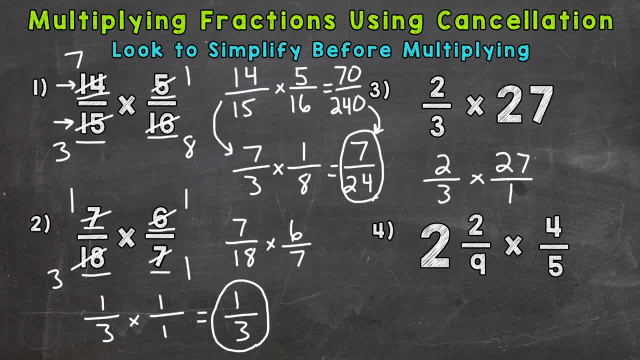 And that's equivalent to 27.. We didn't change the value of 27.. We just converted it to a fraction where we have a numerator and a denominator. So let's see if we have any common factors between our numerators and denominators. And yes, we do 3 and 27 both. 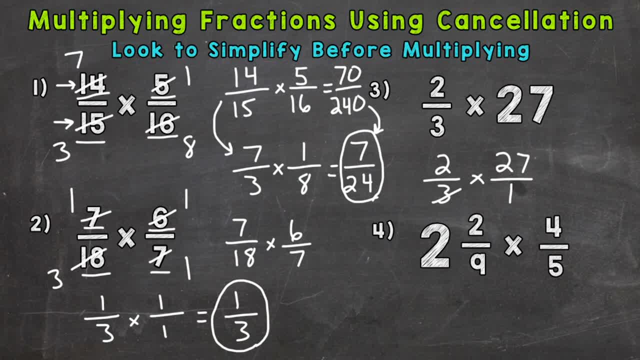 have a common factor of 3.. So let's divide both by 3.. 3 divided by 3 is 1.. 27 divided by 3 is 9.. So let's multiply. Let's multiply straight across: 2 times 9 is 18.. And 1 times 1 is 1.. So we get 18 over. 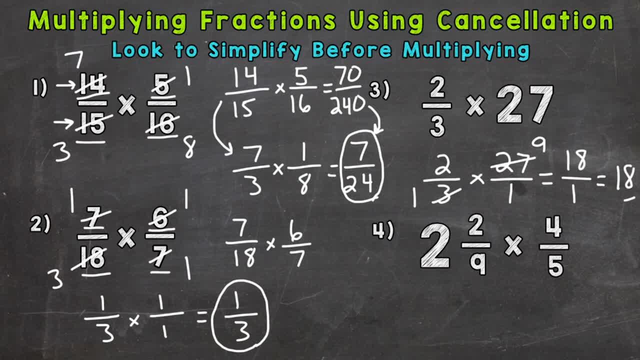 1, which is just 18.. And lastly, number 4, where we have a mixed number times a fraction. So whenever we have a mixed number, we want to convert it to an improper fraction here. So we have a numerator and a denominator And we can do that. 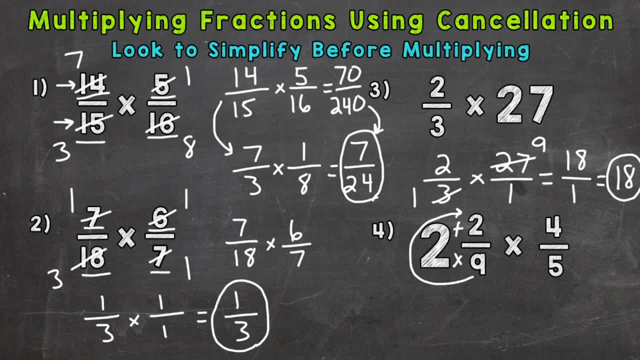 By multiplying and then adding. So multiply the denominator by the whole number. 9 times 2 is 18 plus the numerator of 2.. So again, 9 times 2 is 18 plus 2 gives us 20 ninths. And if you need more help with converting mixed numbers to improper fractions, I'll drop. 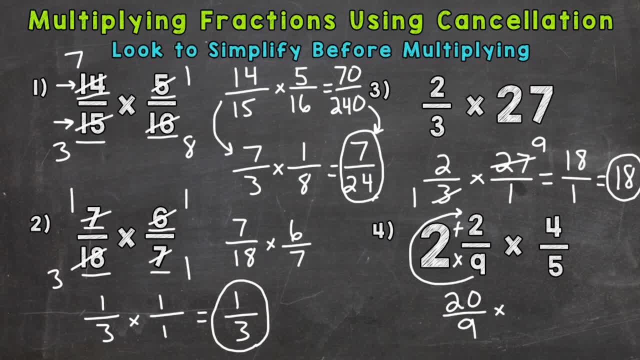 that link down in the description, And 4 fifths we keep as is. So let's see here if we have any common factors between the numerators and the denominators. So 20 and 5 both have a common factor of 5 there. So let's divide 20 and 5 by 5.. 20 divided by 5 is 4. 5 divided.